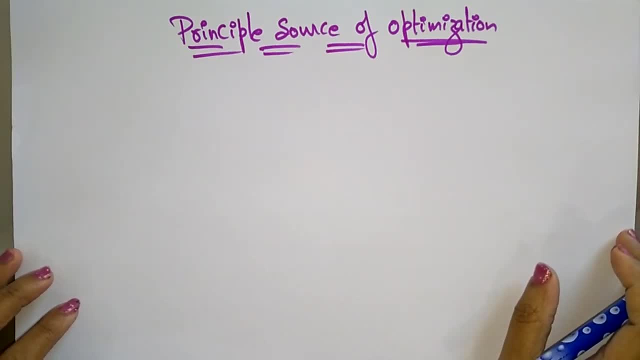 Hi students, welcome back. Coming to the next topic in the subject, compiler design was principal source of optimization. So what is the main principal source of optimization? So this is one of the. the code optimization is one of the level in the compilation process. So this comes under the backend. the code optimization, the code generation and the target machine. This all comes under the backend of the compiler. Now let's see what is the main principal source of optimization. 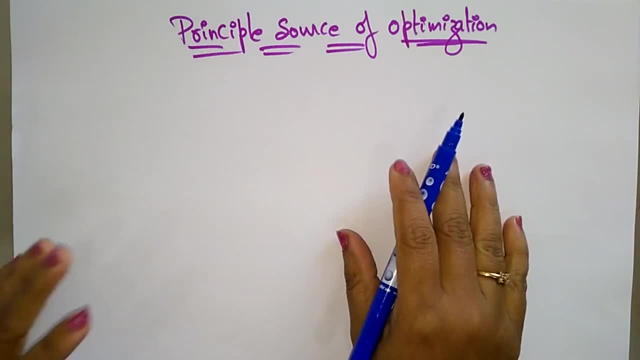 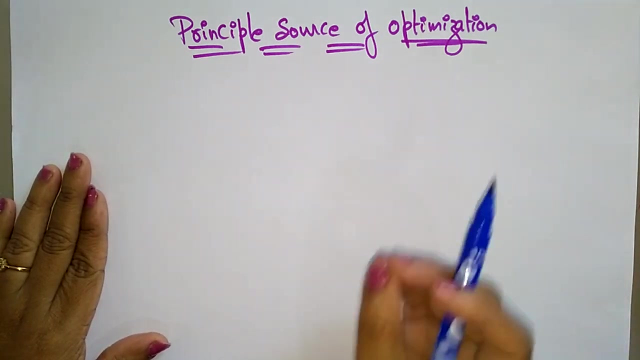 Actually, what is this optimization here? So, whatever the code that want to, produced by the straightforward compiling algorithm, can often be made to run faster or take less space. Okay, so this implement, that is, a straightforward compiling which takes the leg space, is achieved by the program transformations that are traditionally called as optimize. 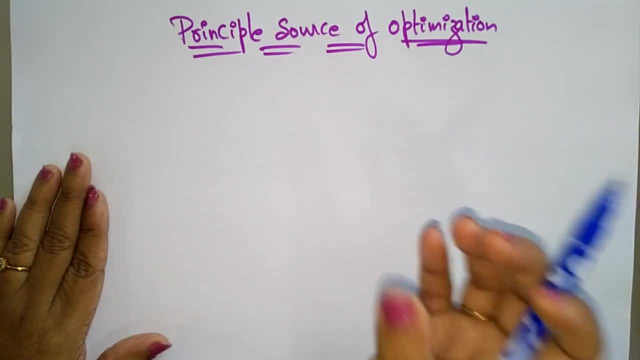 optimization. Okay, so optimizing, you're optimizing the program and you're making to run faster, And the main aim here: you have to take the less space, you have to occupy the less space in the memory. So that is the main concept of optimization: optimizing, reducing and it has to run faster. Now let's see the optimizations There are. the optimizations are classified into two categories. 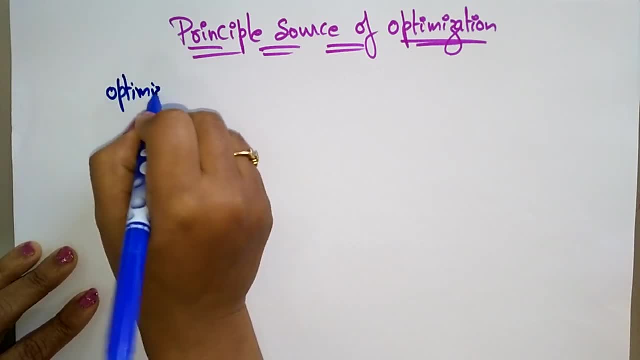 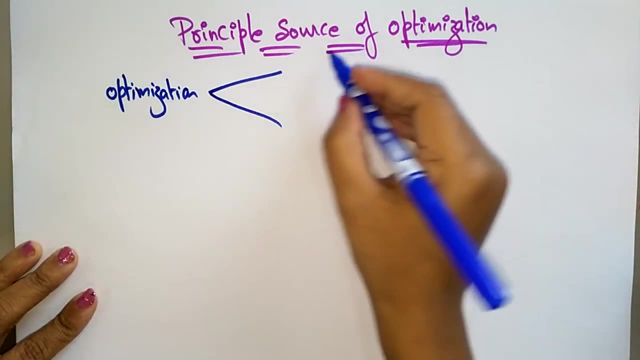 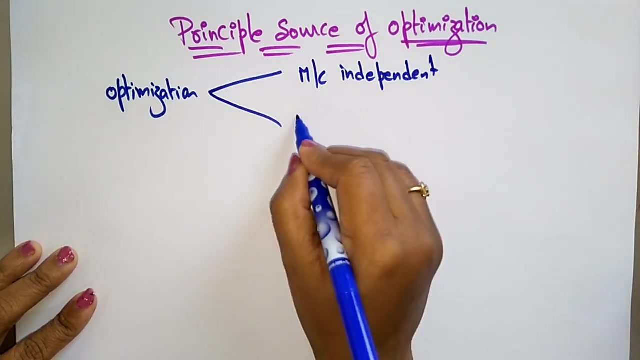 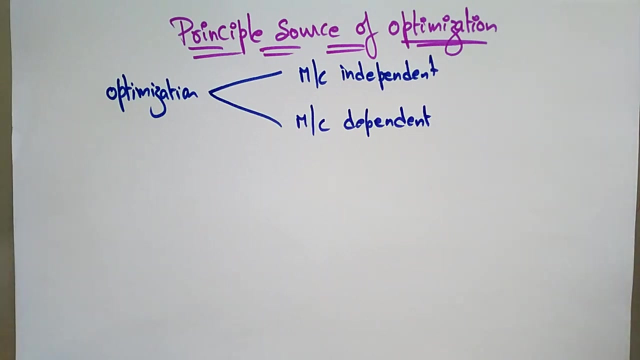 optimization is classified into two categories. So what are the two categories? So one is a machine independent optimization, machine independent optimization and the machine dependent optimization. So if you want to reduce the core and and you want to make the program to run faster, so that can be done. 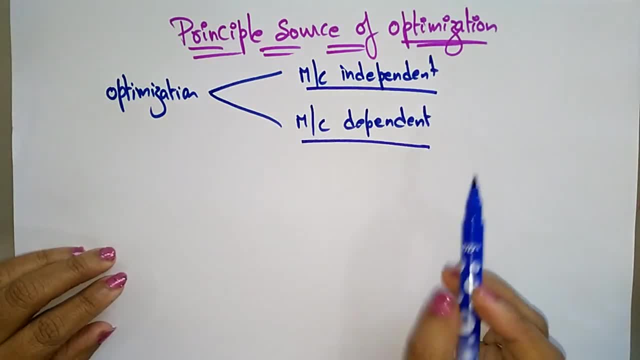 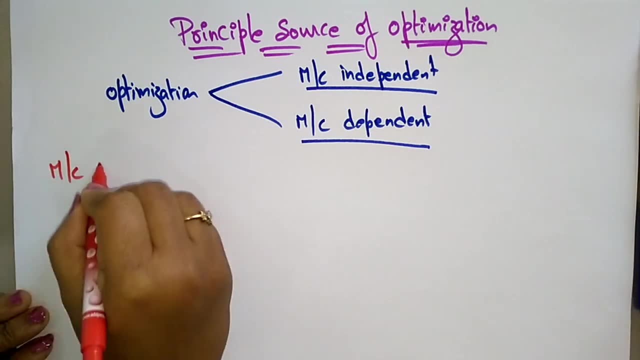 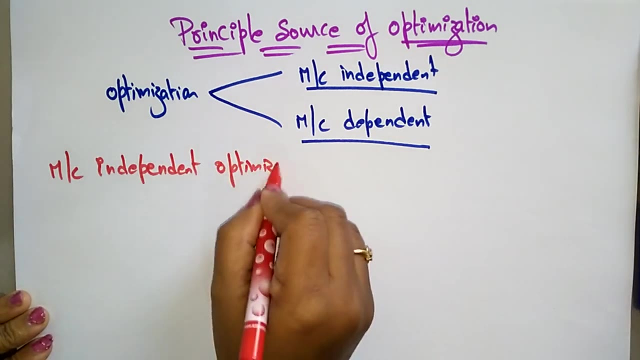 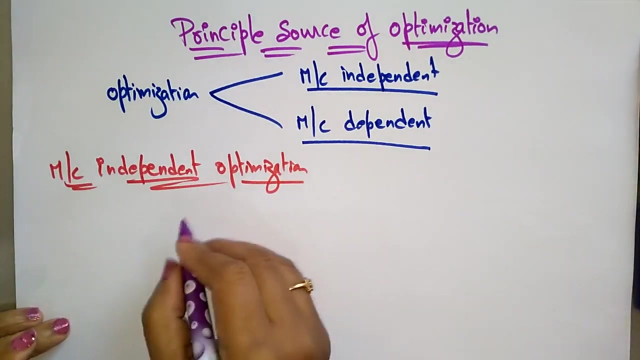 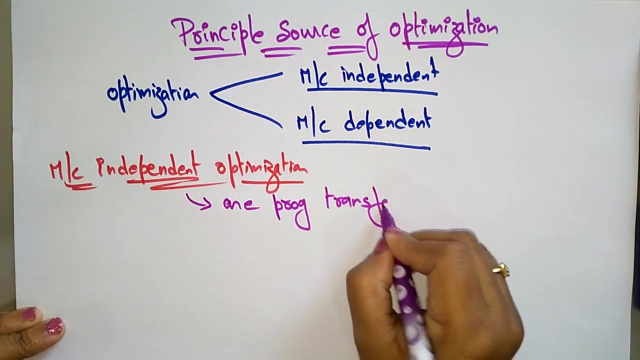 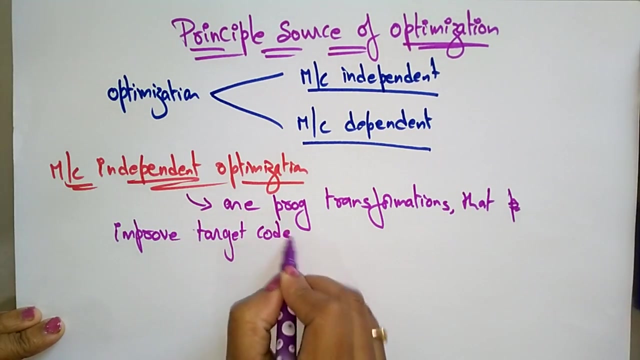 with the help of machine independent or the machine dependent. Now let's see what is this: machine independent optimization, machine independent optimization, So what it means: The machine independent optimizations or program transformations, or program transformations. first let me write, later I'll explain that. improve target code, that improve target code without taking into consideration 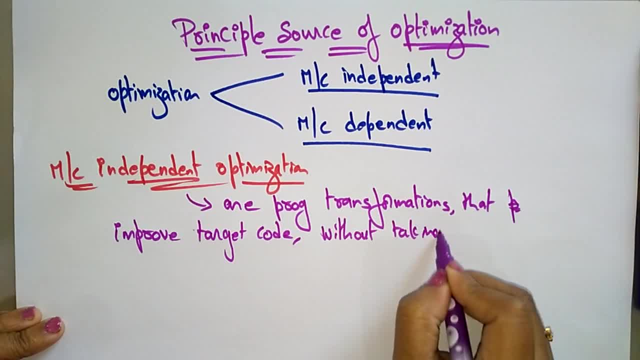 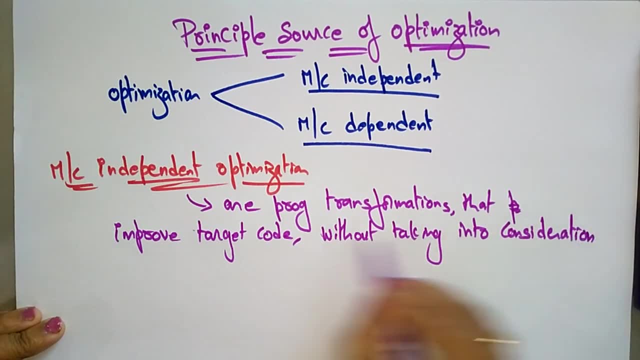 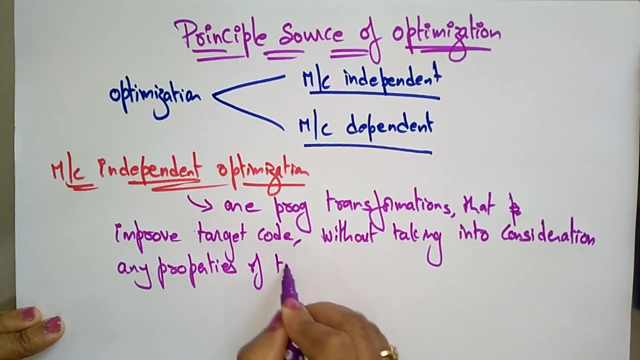 without taking into consideration any properties of target machine, any properties of target machine. so our main aim of using the optimization is to reduce the thing. okay, and you have to make the program as a small and you have to execute it at faster, then what is machine independent? 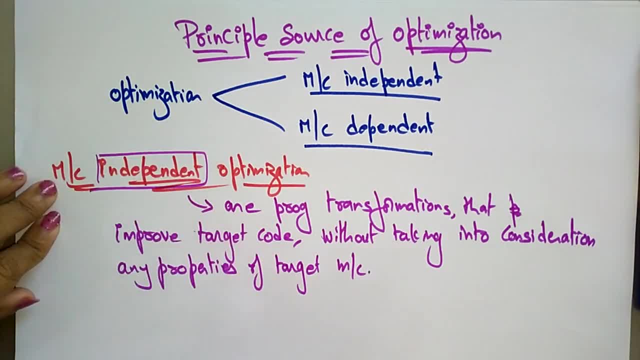 Machine independent optimization. independent, the name itself is saying it is not dependent on anything. so one here the programs machine independent optimization or program transformations. so it is going to transfer the program that improve the target code. so whatever that transformation is going to be done, that improves the target code without taking into consideration any properties of target machine. 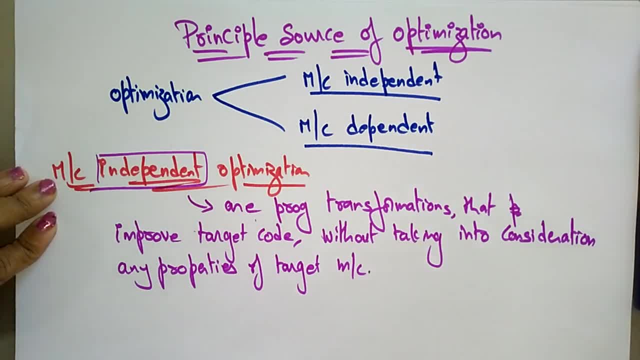 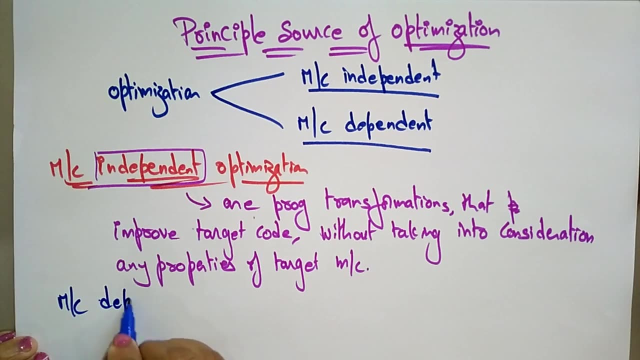 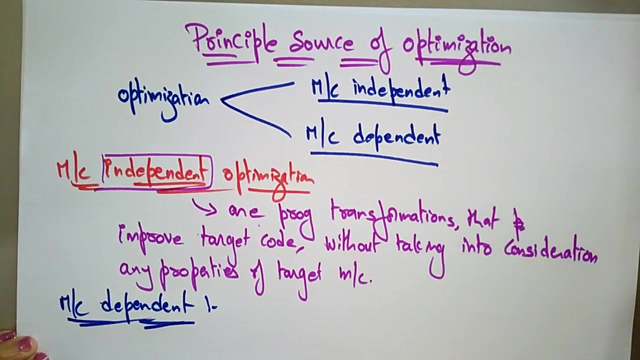 means without taking any help, any Target machine help. it is not taking any target machine help by itself. it is doing, it is transforming the program which improves the target code. then what about the machine dependent optimization? machine dependent optimization, so the machine dependent optimization. here these optimizations are based on register allocation. 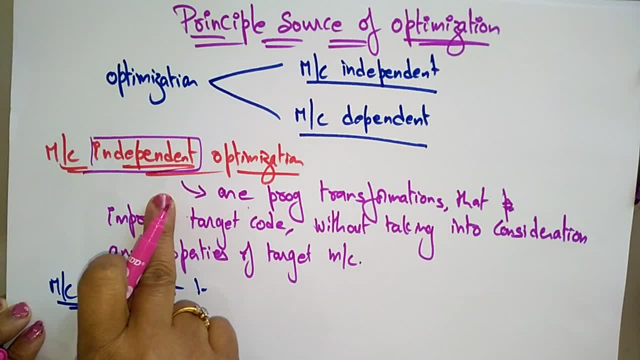 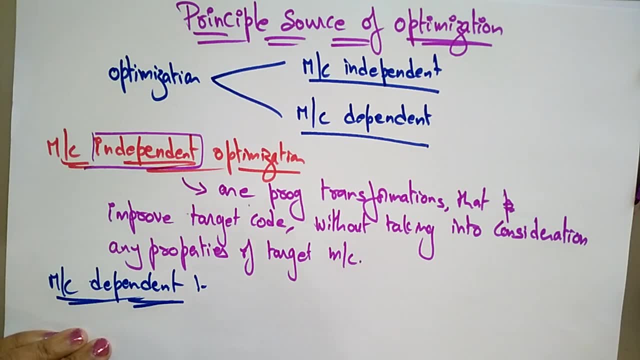 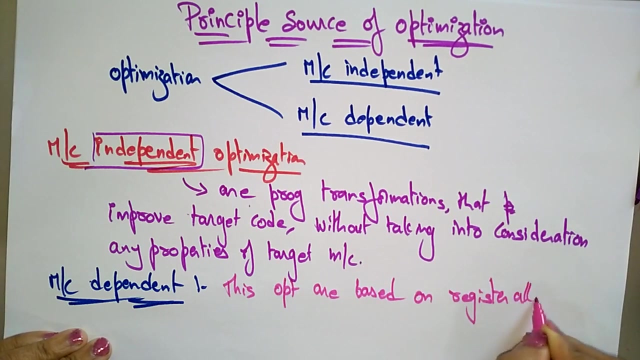 it is depending. the thing is, here is independent, it doesn't bother about any target machine, but here it is dependent. so if it is dependent means it has to use some components that uh, in the memory. okay, so this optimization or based on register allocation: register allocation and utilization of special machine instructions.